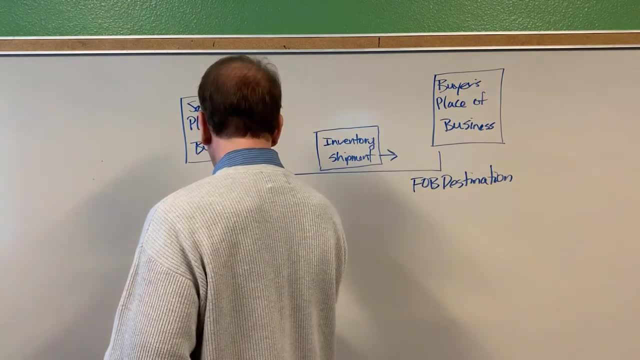 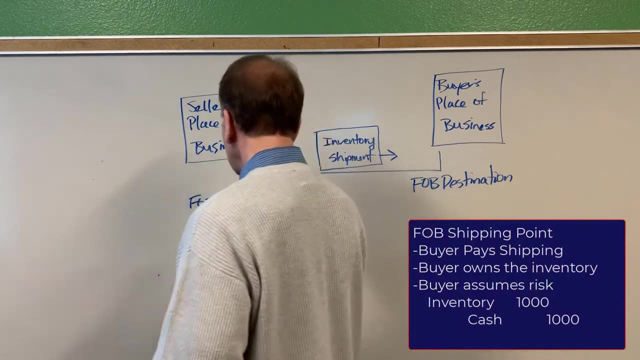 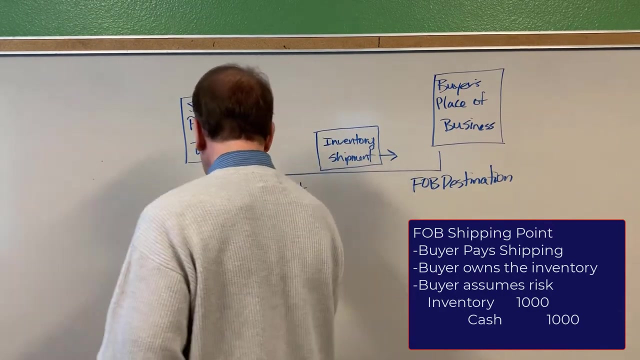 the inventory. So basically, what's happening then is the buyer pays the shipping During transit. well, they're paying the shipping, The buyer owns it during transit. The buyer assumes the risk of the inventory, So they want to make sure that they properly. 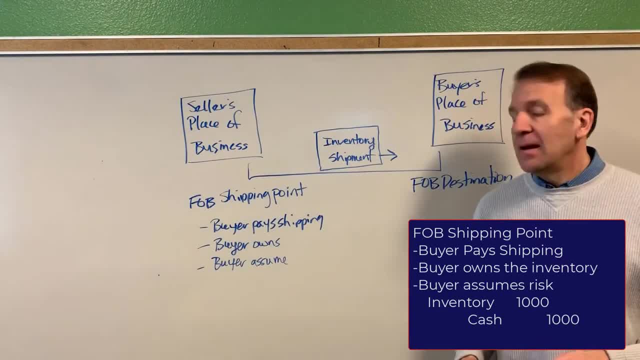 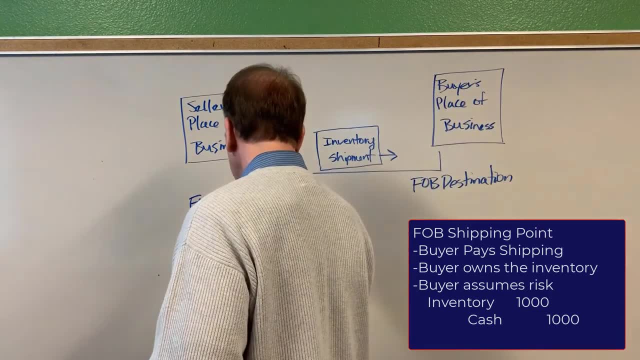 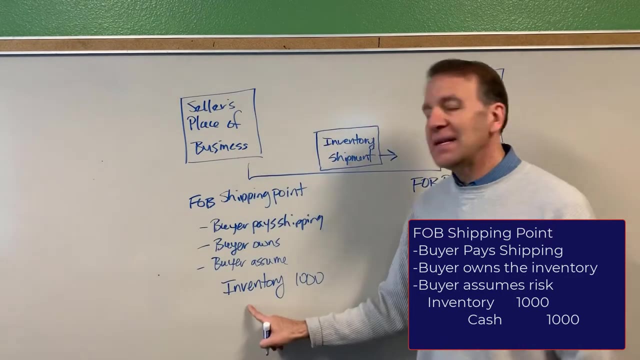 insure it. Okay, Now the journal entry is a little bit different. The journal entry: let's say we're paying a thousand dollars for this shipping. Well, the shipping cost will be attached to the inventory itself. It will be included with the. 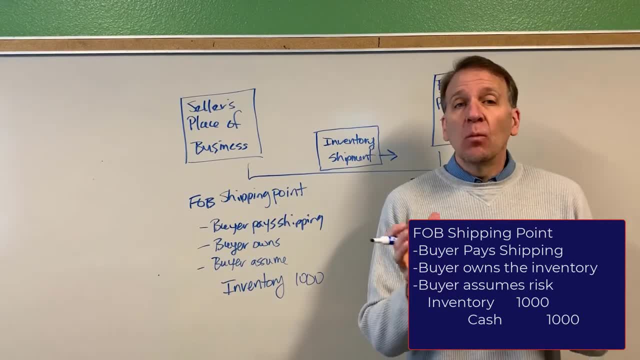 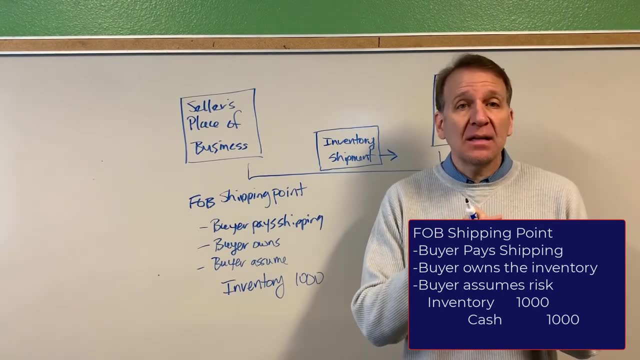 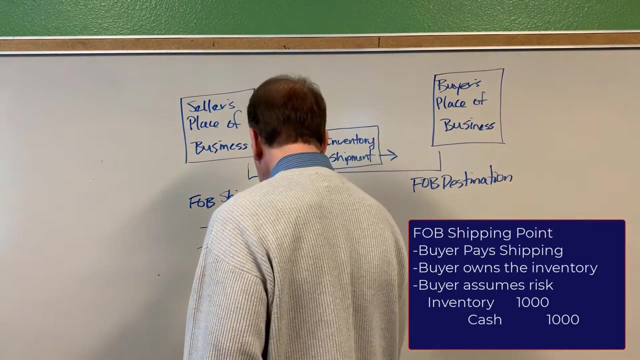 inventory. Whenever we're purchasing inventory, what goes into that inventory cost isn't just the price of the inventory. It's also any shipping costs, taxes, tariffs, you know, any other costs that are incurred, get attached or included with the inventory. So here's our 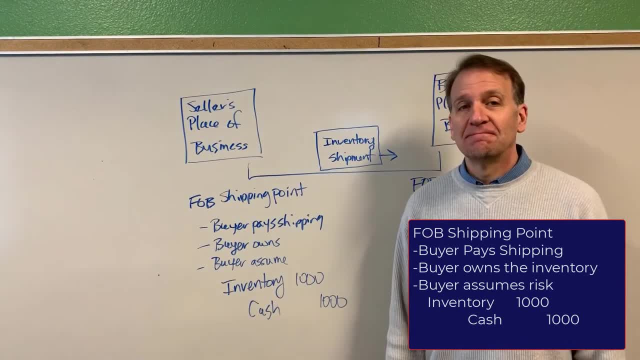 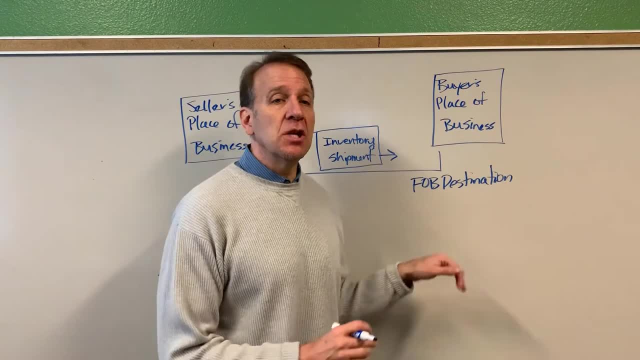 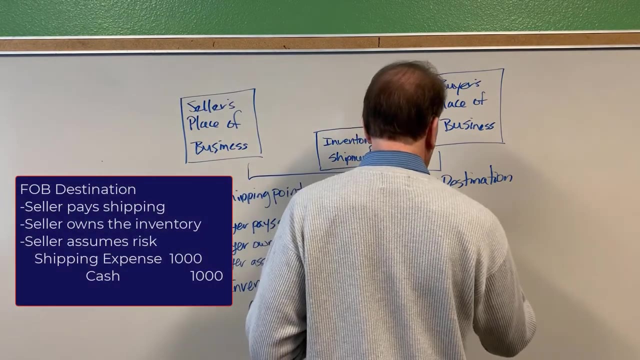 budget: agent number 10, 40 days, going to be sold. Applause: likeHello NASA. Let's go ahead and get that hundred dollar bill. So here's our destination and it's going to go into inventory. Now let's take a look at. 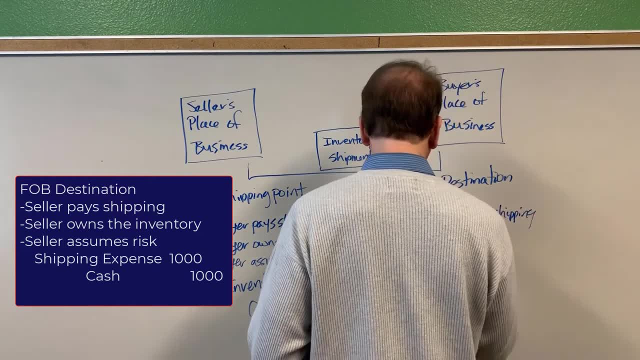 what happens if this is FOB destination? If this is shipped FOB destination, then this stuff here is kind of the opposite. What's happening is the seller pays the shipping, The seller owns, and I'll put пmarang scene: Sau-design a slide without binges. 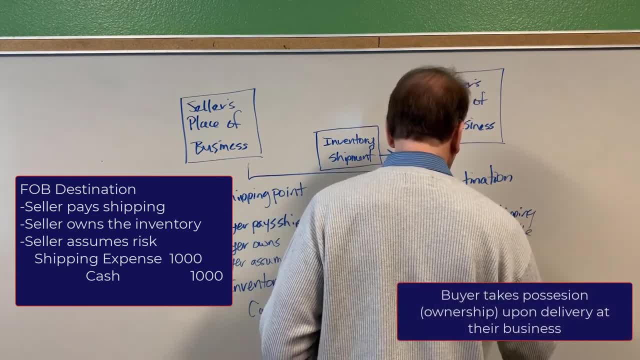 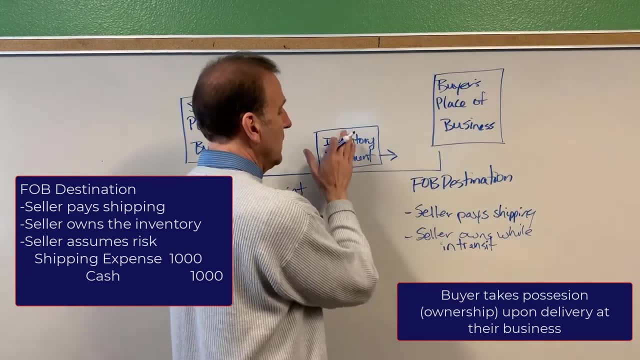 down here while in transit. Transit is some På humblelinear by Course. in our website, режим 사udingпôm daredå. Transit just means while it's being shipped. okay, So it's in transit right here. So if it's FOB destination, the seller's paid the shipping. 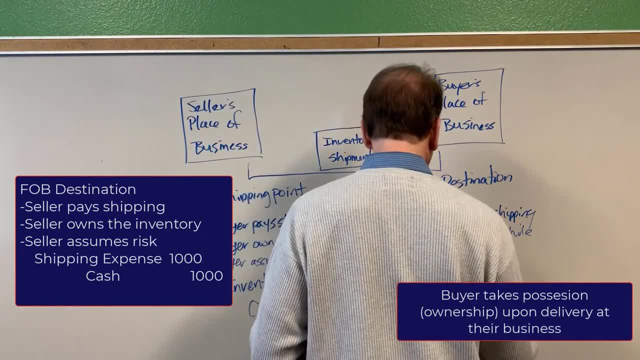 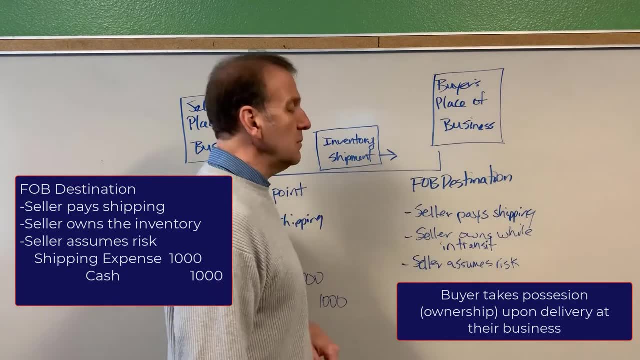 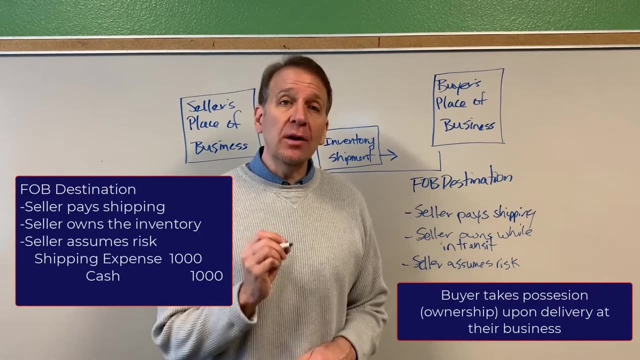 the seller owns it and the seller assumes all risk, So they want to make sure that they have it properly insured. Now let's take a look at the journal entry for that $1,000 payment- If the seller is paying the shipping. 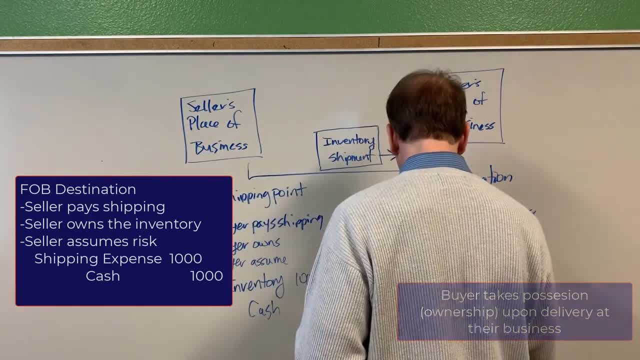 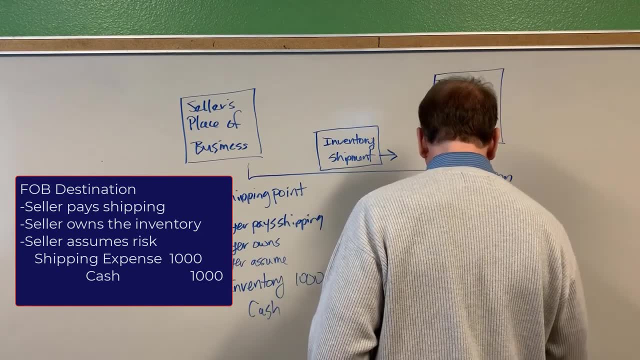 then they're going to debit shipping expense, or you might call it freight expense, And we said that it was $1,000. And then if they paid it it would be a credit to cash, okay, So notice the difference here.